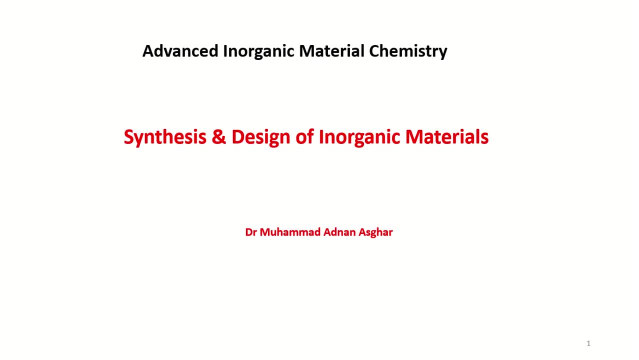 Bismillah ar-Rahman ar-Rahim, Assalamu alaikum, dear student, My name is Dr Muhammad Adnan Asghar and today the topic of our discussion is synthesis and design of inorganic materials under the subject of advanced inorganic material chemistry. 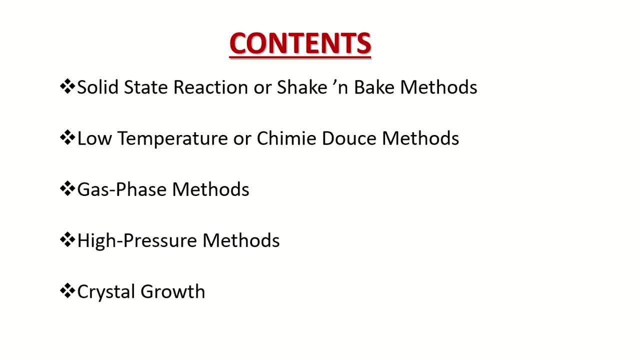 Here are the contents of the lectures that is delivered. that is going to be delivered in some parts. The first is the method that, that is, we are going to use for the synthesis and fabrication of inorganic material. is the solid state reaction or shake and bake methods? 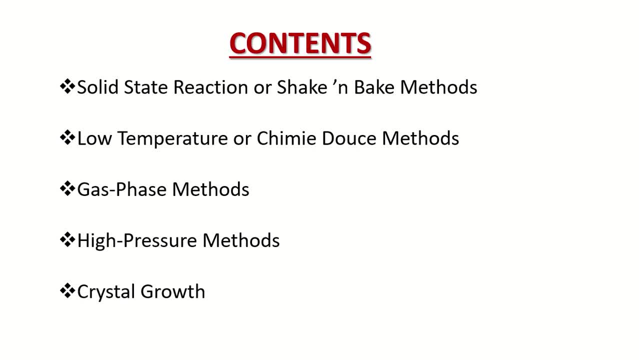 The second would be the low temperature or chymidose methods, While the third one is gas phase methods. Fourth one is high pressure methods and the last one that we will discuss in our next lectures is the crystal growth methods for the synthesis and fabrication of inorganic materials. 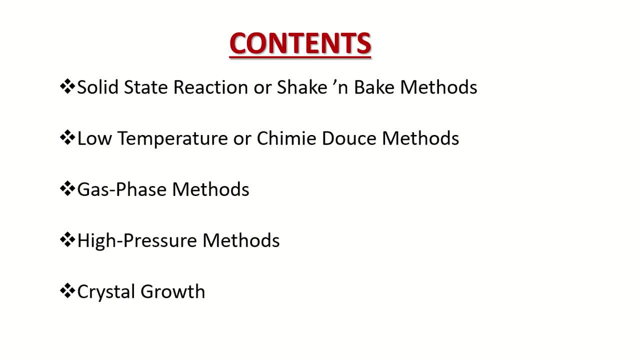 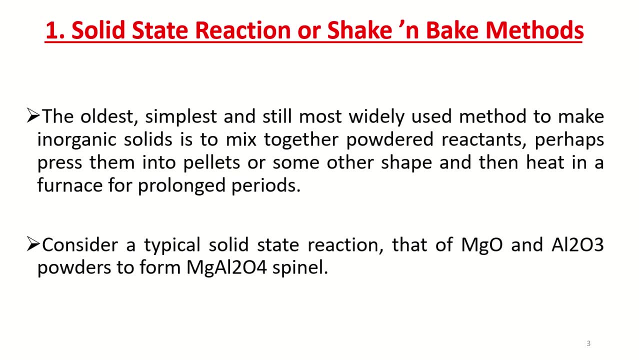 So let's talk about the solid state reactions or shake and bake methods. Many methods can be used to synthesize non-molecular, inorganic solids. Some solids can be prepared by a variety of routes, but others, especially those that are not thermodynamically stable, 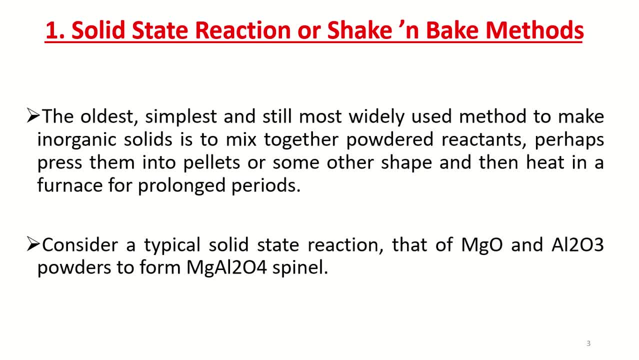 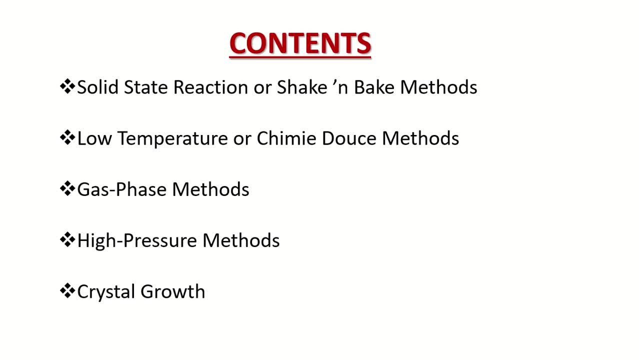 Maybe much more difficult to prepare And may require special methods. So here are the different methods that we are going to discuss. Non-molecular inorganic solids can also be synthesized in various forms, For example in as a fibers, films, forms ceramics. 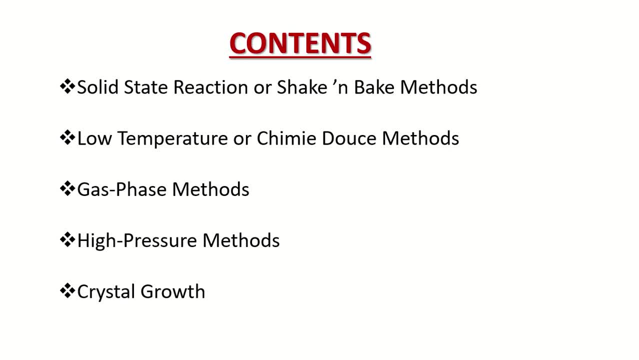 powders, nanoparticles and single crystals. For these different forms, Synthesis is not a big problem. Instead, It is the optimization of the processing and the fabrication procedures that is crucially important. So it means that we the synthesis of different inorganic materials is actually a not a big challenge. 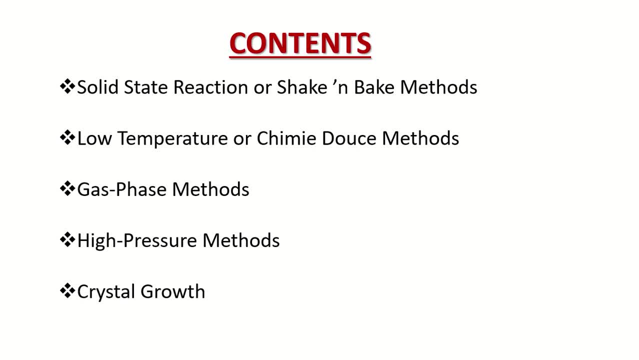 But the challenge is actually the optimization of the conditions for the perfect synthesis of inorganic materials. For example, if a compound crystallize in the form of crystals, So we need to prepare The crystals in a very smooth way, because if the crystal have some of the cracks, are some impurities adsorbed on the surface of the crystals, then it may affect the characteristics properties of the particular material. 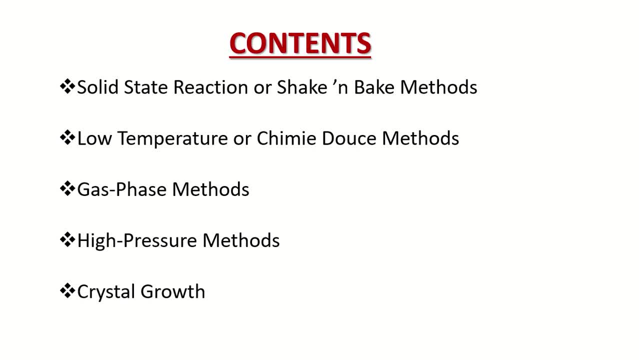 So the best method is actually to find out the optimized way for the processing and the fabrication of that particular material. This link to the possibilities of doping, modification of properties and possibilities for new type of applications, which makes the study of inorganic solids. 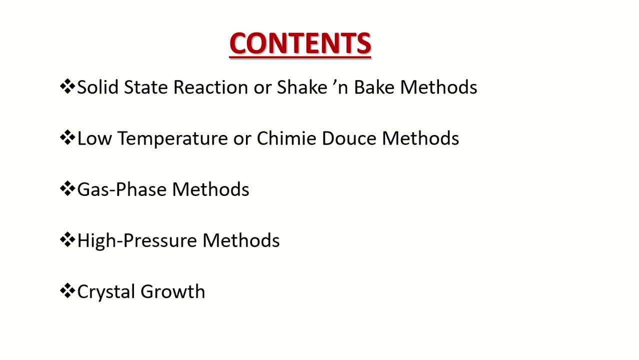 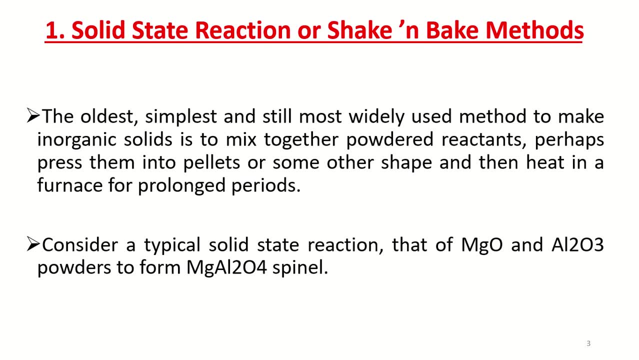 Such as diverse, challenging and stimulating area of science, Science. In this lecture, the main methods used to synthesize inorganic solids would be summarized Together with the method used to fabricate solids in different forms. A few new materials will be introduced, such as amorphous silicon and diamond films. 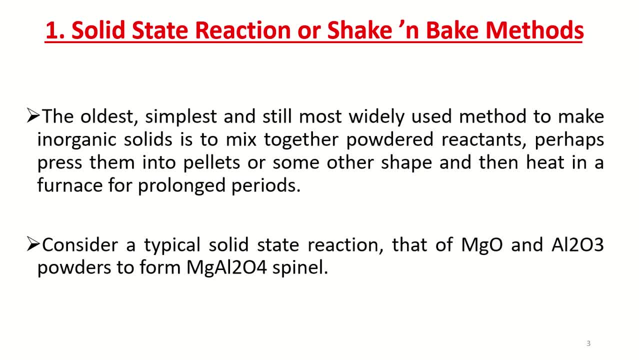 Which are very important, Technologically important, and we will discuss easily within the framework of this synthesis methods. So it is quite obvious to understand that actually the synthesis of the material is not a big challenge, But actually the challenge is the optimization of the conditions at which a perfect material can be. 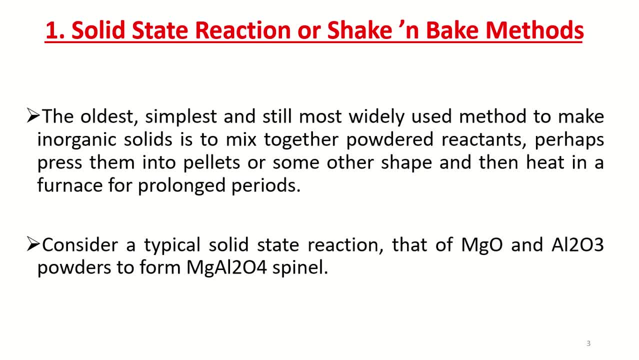 Harvested, So this is actually the best way to treat with the materials. The first is actually the solid state action, or sometime known as shake and bake methods. This is actually the oldest, simplest and still most widely used method to synthesize inorganic solid is to mix together powdered reactants. 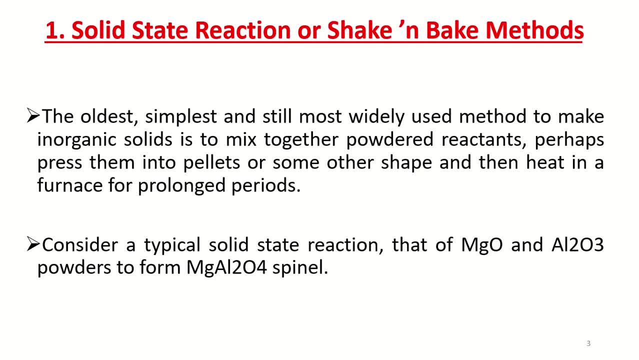 But the most common method to synthesize inorganic solids Is to mix together powdered reactants, Perhaps press them into the perfect pallets or some other shape, And then heat in the furnace for prolonged periods. The method is not so sophisticated, Hence the use of alternative names such as shake and bake or beat and heat. 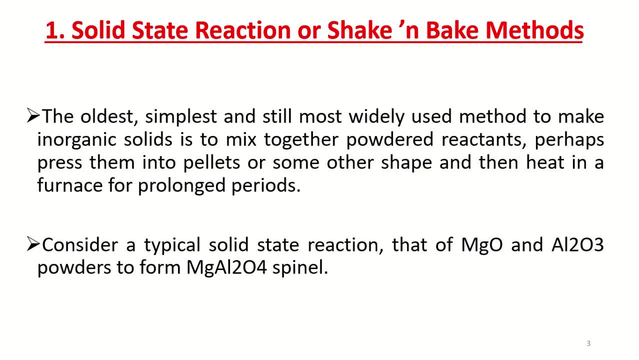 It is nevertheless very effective And, for example, Almost All the high curie temperature superconductors Were first prepared by this method. So it is For most used method and it is supposed to be the oldest and the simplest method to synthesize high quality and high applicable materials. 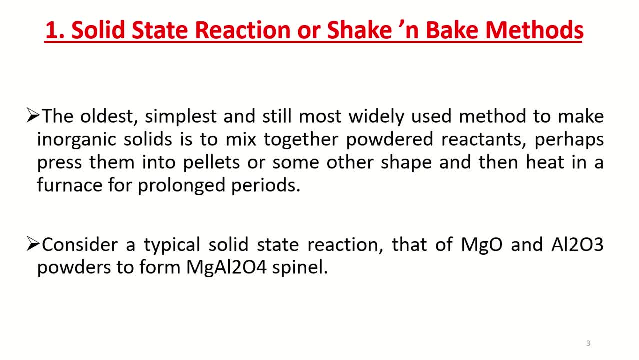 For example, The High curie temperature superconductors, are actually first prepared by using this method. Solid state reactions are Drastically slow because, Although the reactants may be well mixed At the level of individual particles- Individual particles, For example. 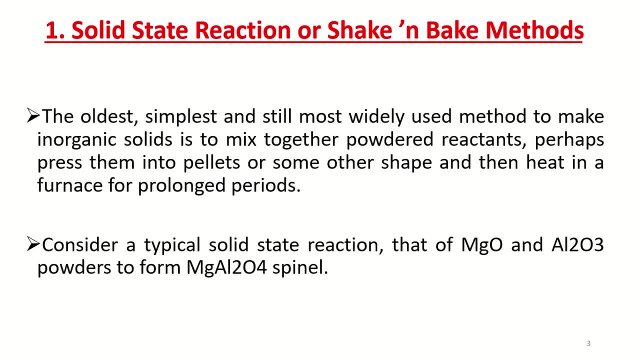 On a scale of one micrometer, or sometimes tens per minus Three millimeter. On the atomic level, They are very inhomogeneous. In order to achieve atomic level, mixing of reactants, Either solid state counter, diffusion of ions Between Different particles. 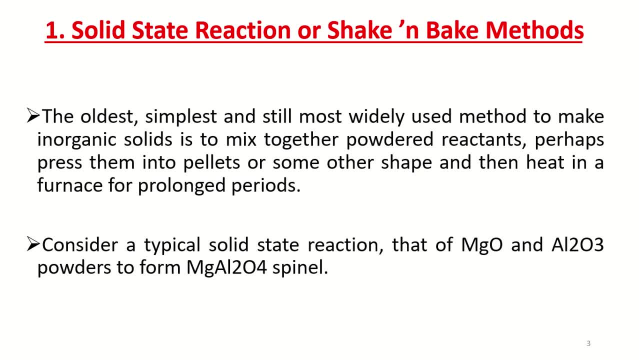 Or liquid Or gas Phase. Transport Is Quite necessary To bring together atoms of Different elements And, in correct ratio, To form the desired product. So it is very important to Mix the Reactants in a exact 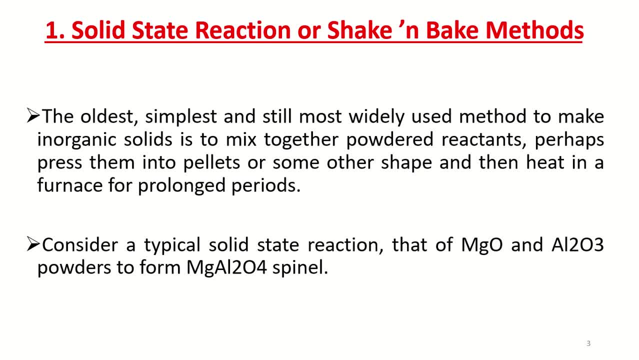 Ratio To To get the best Desired Product. For example, Consider A typical Solid state Reaction, That Of Magnesium Oxide And Aluminium Oxide, Al2.. O3. Powders. 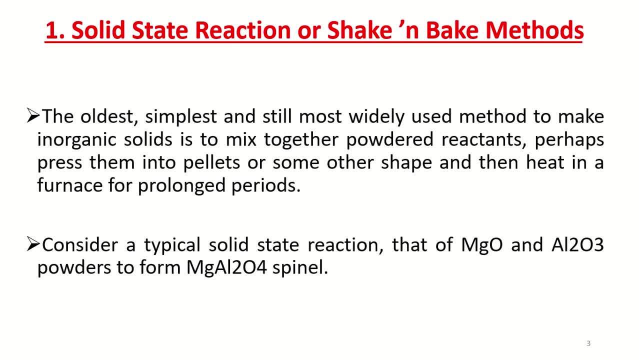 To form: Magnesium, Aluminium Oxide, Mg, Al2. O, 4. Spinal. Okay, So Let us Consider The Various Processes Involved In this Reaction, And It is. 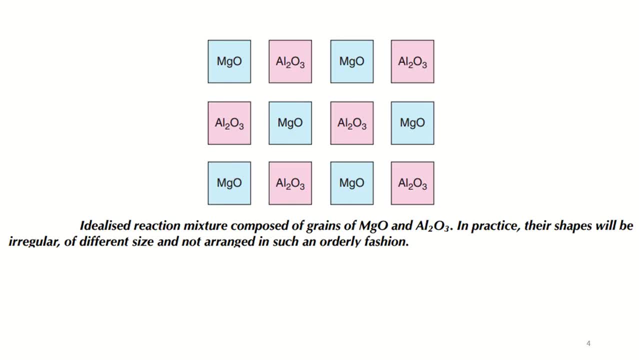 Actually Shown In this Diagram: Idealized Reaction Mixture Composed Of Grains Of Magnesium Oxide And Aluminium Oxide. In practice, Their Shapes In an 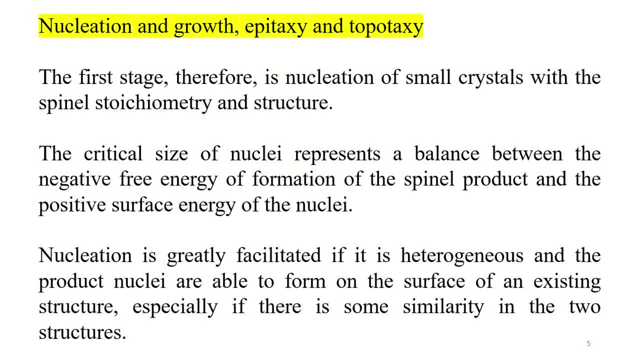 Order, Fashion. So Nucleation, How It Happens, Nucleation And Growth, Epitaxy And Topotaxy At Every Interface Between Contacting Grains Of 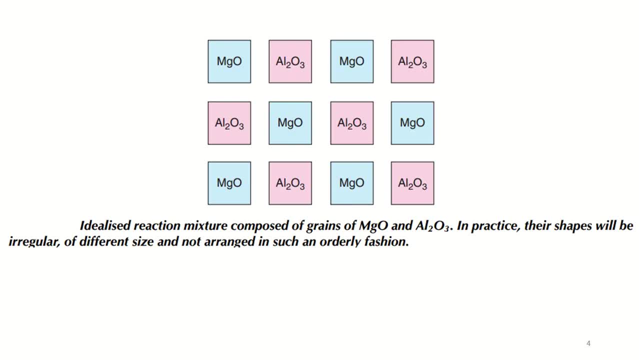 Magnesium Oxide And Aluminium Oxide. Magnesium Oxide: All The Ingredients Necessary To Form The Magnesium Mg Al2O4.. Product Are Present. The 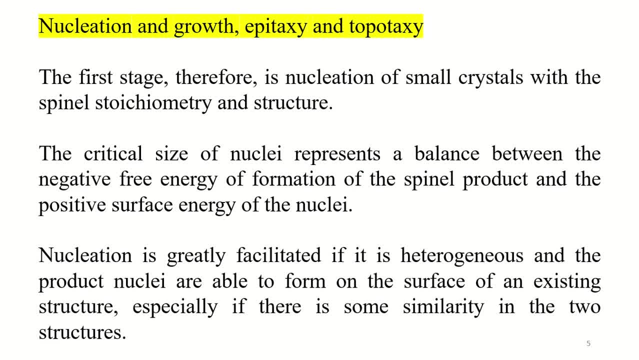 First Stage Therefore. Therefore, Is Nucleation Of Small Crystals With The Spinal Stitiometry And Structure For The Form Of Magnesium And Not 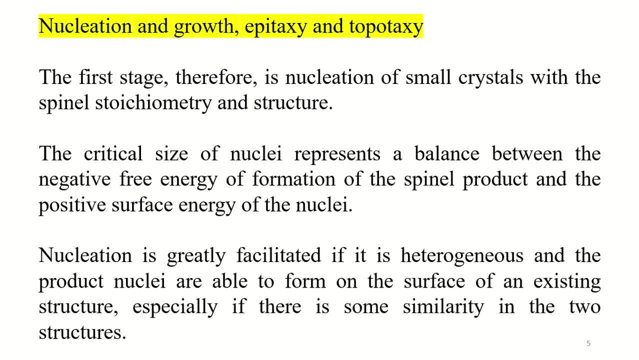 To Disintegrate Spontaneously. As Soon As They Form, They Must Usually Be Several Tens Of Angstrom Across, That Is It Should Be They. 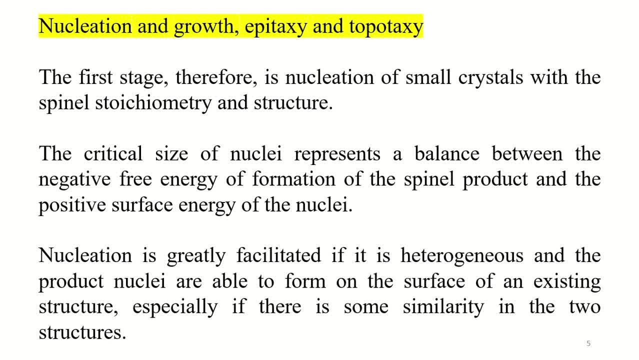 Must Be For The Size Of Nuclei Represents A Balance Between The Negative Free Energy Of Formation Of Spinal Product And The Positive Surface. 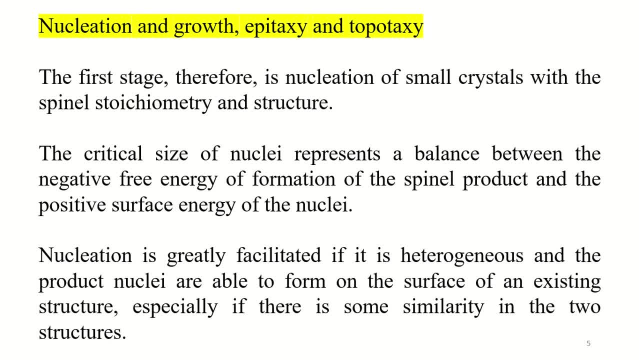 Energy Of Nuclei. If The Nuclei Are Small In Size, Then The Surface Area To The Volume Ratio Is Supposed To Be Too. 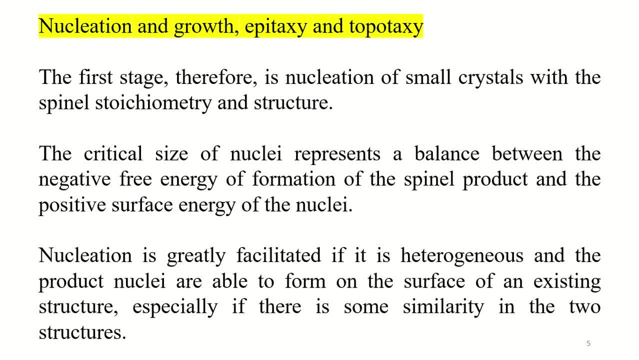 Large And Nuclei Are Small In Size, Then The Surface Area To Be Large And Nuclei Would Be Unstable. Nucleation Tends To. 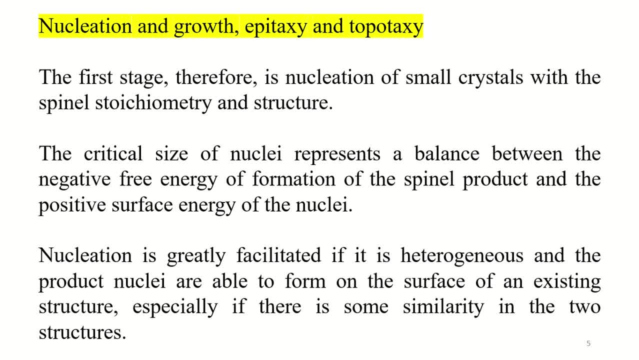 Be More Difficult, Simply Because Of The Large Number Of Ions That Must Get Together In Correct Arrangement To Form If It Is Heterogeneous. 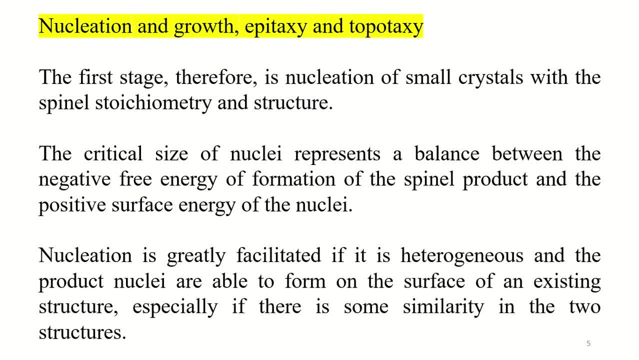 And The Product Nuclei Are Able To Form On The Surface Of An Existing Structure, Especially If There Is Some Similarity In The Two. 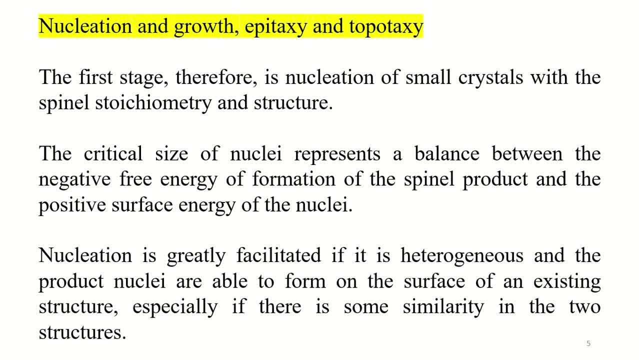 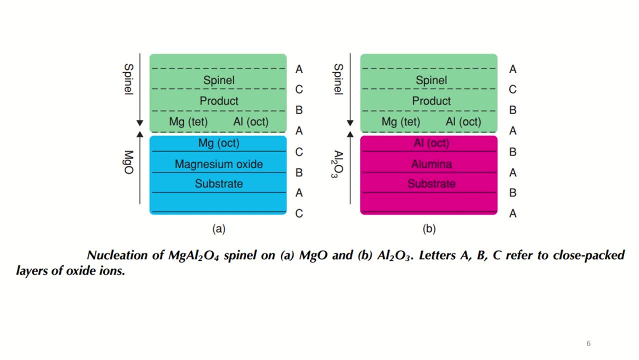 Structures So To Form On The Surface Of An Existing Structure, For Example The Magnesium Oxide And Aluminium Oxide, Mg O, Al2O3. Reaction. 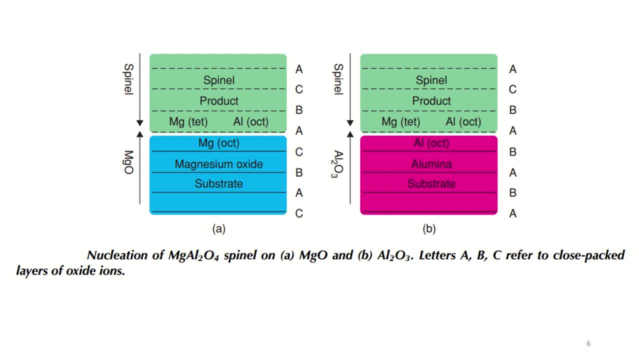 To Form Spinal. Provides Two Examples Of Possible Magnesium Oxide Grains As Shown In This Picture, At The Magnesium Oxide And Magnesium. 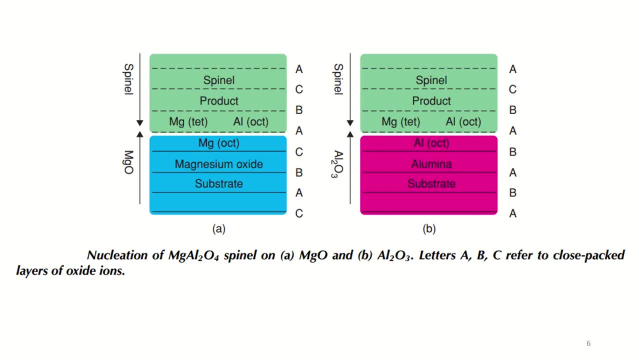 Aluminium Oxide Interface, Provided That Magnesium Aluminium Oxide Nucleus And Underlying Magnesium Oxide Are In Continued Unchained, Since It Is Ccp. 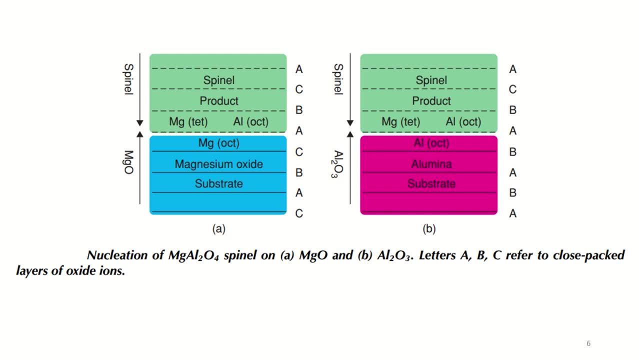 In Both Structures, Where As Within A, B, C Stacking Sequence As Shown In This Figure A A Part Of This Figure In The Octahedral. 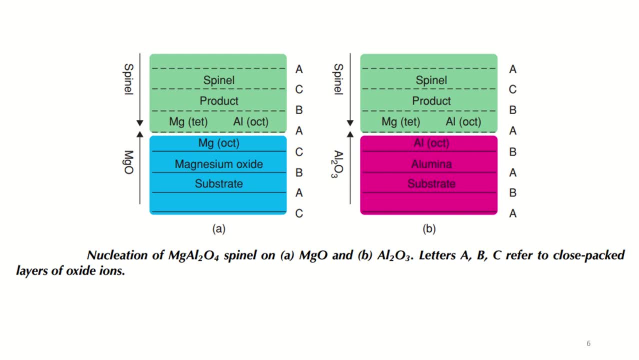 Sides, Octahedral Sides, The, For Example, For The Rock Salt Structure, Whereas In Spinal Magnesium Occupies One Eighth Of The Tetrahedral. 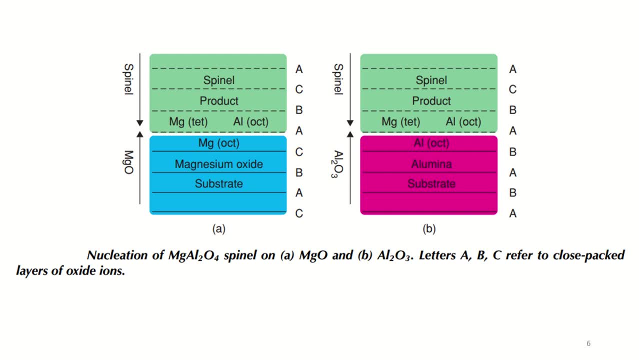 Sides, With Aluminium In The Half Of Spinal Nucleus On Top Of A Magnesium Oxide Structure, And That Magnesium Oxide Structure Would 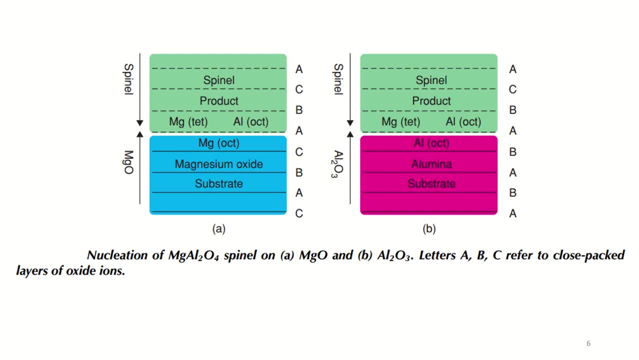 Also Considered As Substrate, Is Relatively Easy Because Of The Structure Similarity Of Magnesium Oxide Nucleus With A Huge Or Large Surface. 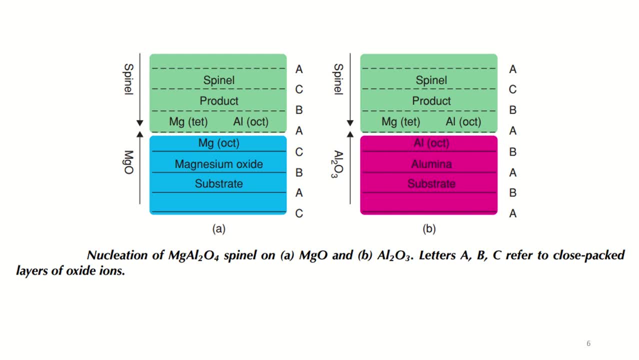 Area At A Suitable Oriented Aluminium Oxide Al2O3.. Slash Magnesium Aluminium Oxide Interface. The Situation Is Quite Similar, But Now The Oxygen. 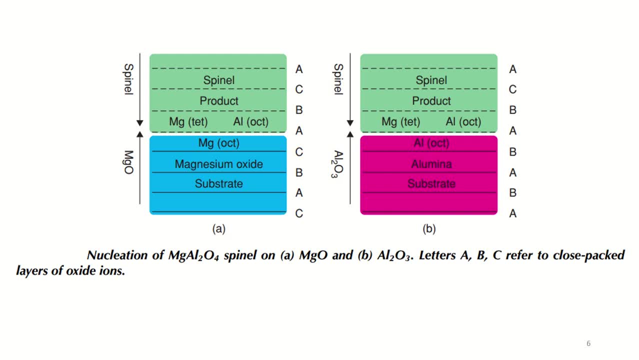 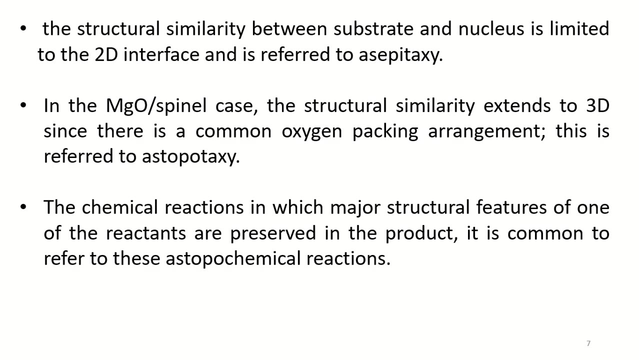 Aluminium Oxide To Ccp In Spinal Spinal Means. The Aluminium Oxide Has The Corundum Structure With Hcp, Oxide Ions And Aluminium. 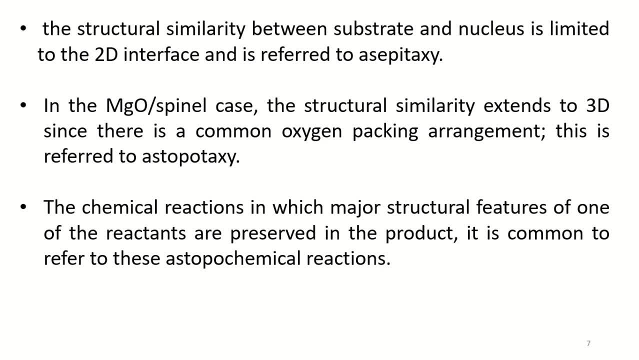 In Two Thirds Of The Octahedral Sides. Actually, Orientation On Aluminia Substrate Is Still Easy, But The Structural Similarity Between Substrate 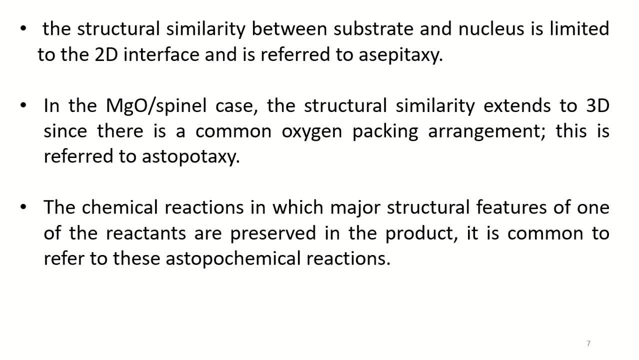 And Nucleus Is Quite Limited To The Two Dimensional Interface And Referred As Epitaxy In Magnesium Oxide To Three Dimensional Since. 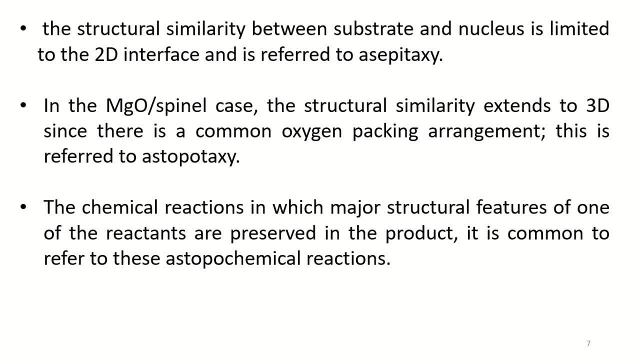 There Is A Common Oxygen Packing Arrangement. This Is Referred To Topotaxy When Discussing The Chemical Reactions In Which Major Structural Features Of 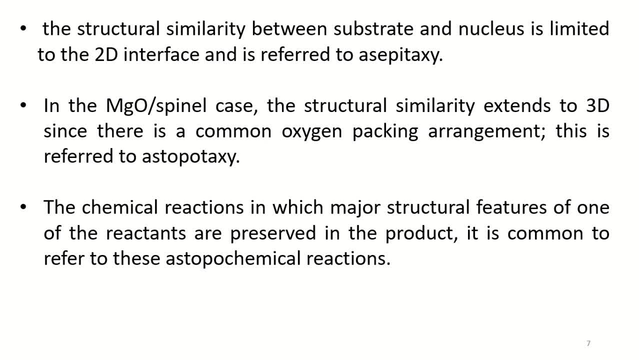 One Of The Topo Chemical Reactions. Epi Tactic And Topo Tactic Features Are Common In Solid State Reactions In Crystal Growth And 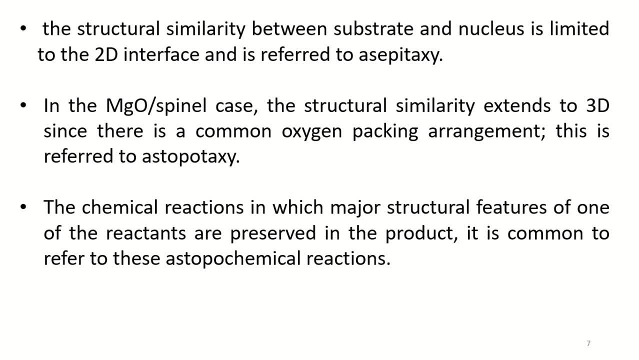 Oriented Thin Film Depositions And An Interclation Reactions And Phase Transitions Are Quite Common In The Side. Reactions In Phase Transitions. 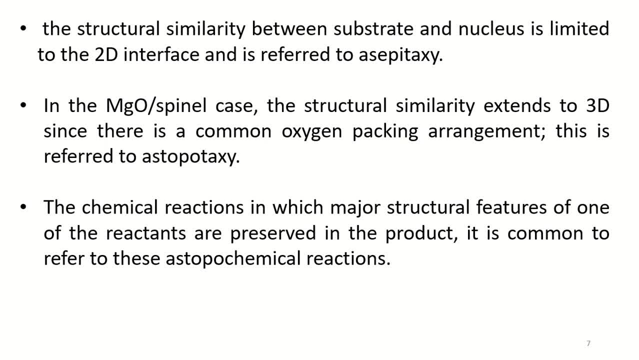 We Know That The Phase Transition Is Actually The Transformation Of A Phase From Any Compound To A Side And So On, But In Solid State. 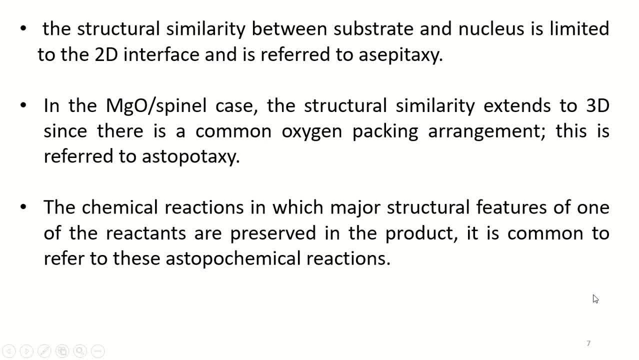 Transitions. We Have To Let You Know That Solid To Solid Phase Transitions Is Actually The Transformation Of One Solid Form Of A Common Interface. 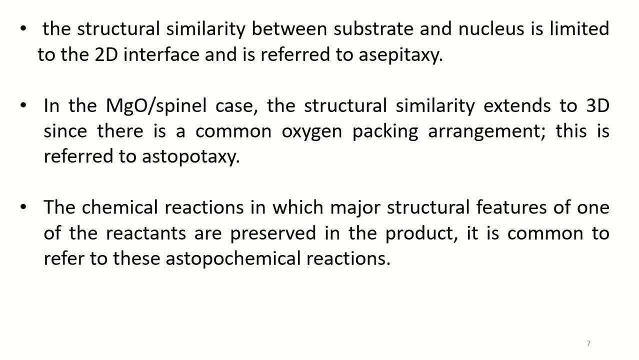 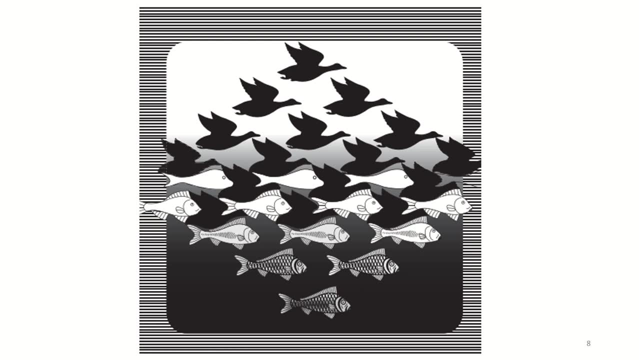 May Have Very Different Properties And Can Transform In Per Capability From One To Another. A Beautiful Analog Is Supposed To Be Provided By The 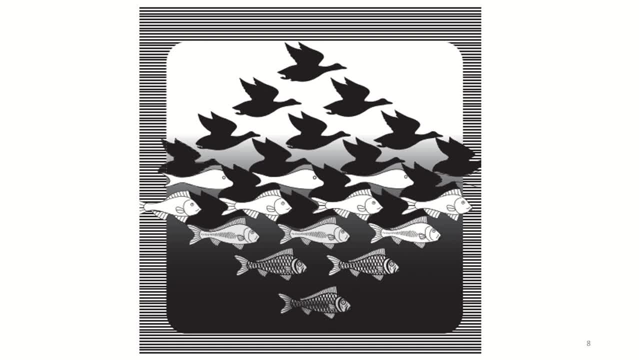 Structure In The Cross Over Region. The Structure Has Recognizable Features Of Both Fishes And Birds, But It Is Not Completely One Or The Other. 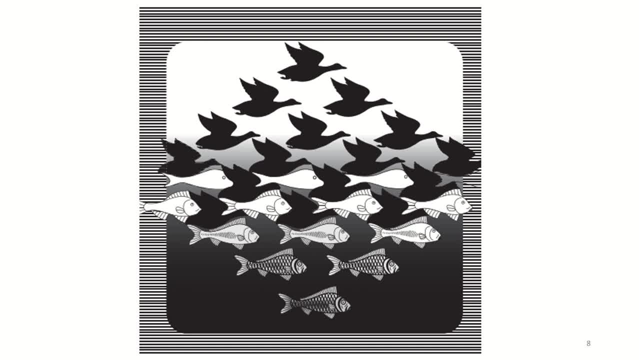 Similar Effects May Occur At Interface. The Coordination Environment Of Atoms At Interface Are Different To Other Side Of The Interface. In Practice Atomic 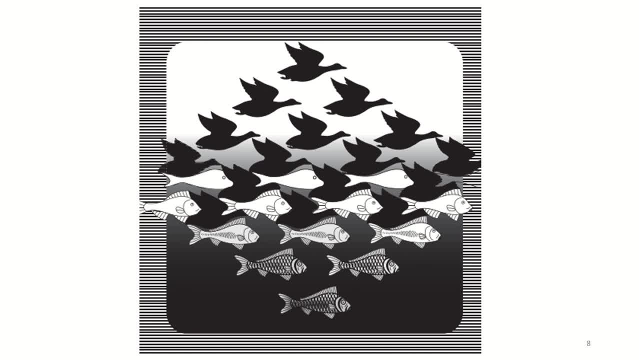 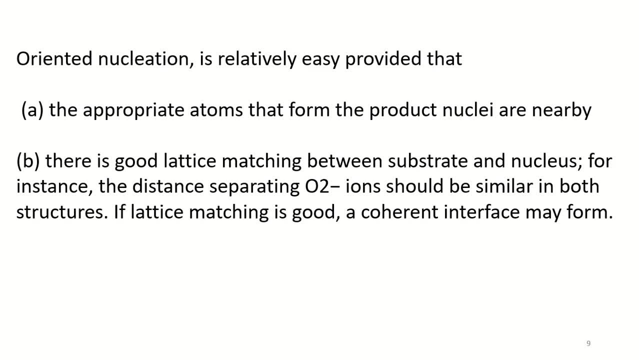 Displacements May Also Occur Further. Complicating The Structure Details Within Nucleation Of The Kind Described Above Is Relatively Easy, Provided That A 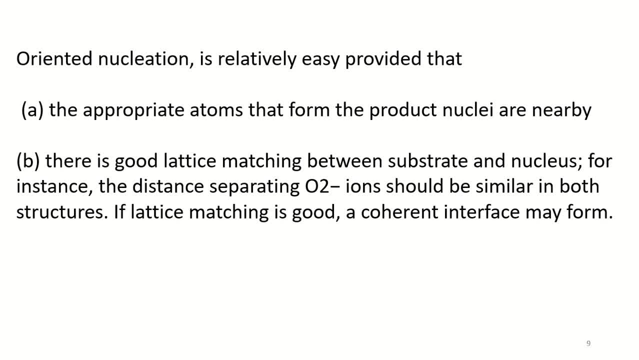 If Appropriate Atoms That Form The Product Nuclei Are Nearby And There Is A Good Latest Matching Between Two Minus Ions Should Be. 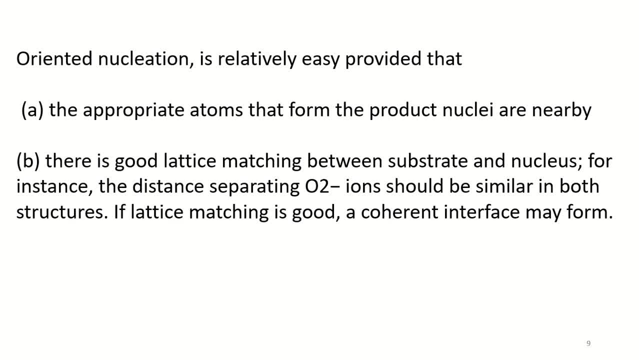 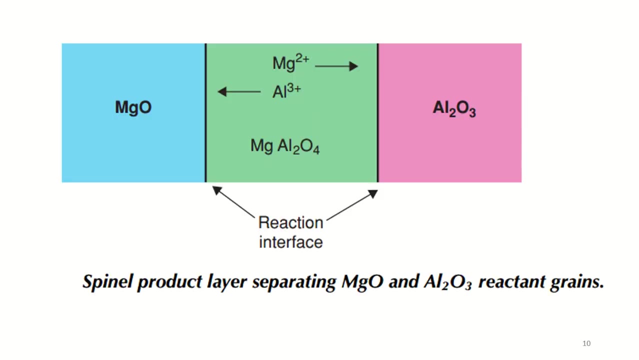 Similar In Both Structures. If Latest Matching Is Good, A Coherent Interface May Form. If Latest Matching Is Not Good, Then The Large Strains Hatch. 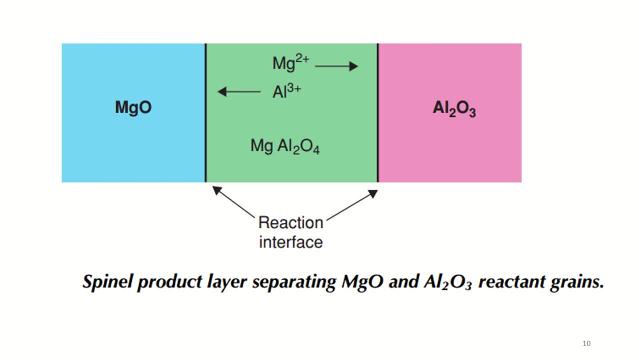 From The Substrate In Our Magnesium Oxide And Aluminium Oxide Reaction Mixture. As We Can See In This Picture, We May Expect Thin. 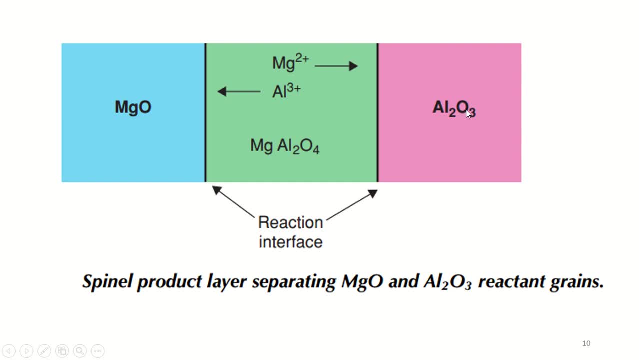 Nuclei Of Spinal To Form Touching, Because All These Three Structures Have Close Packed Oxide Arrangement And Latest Matching Across The Interface. 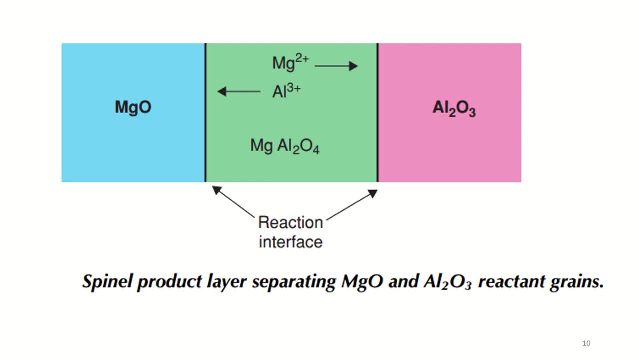 Should Be Very Good, Although The First Few Atomic Layers Of Product Nuclei Is More Difficult Because Effectively, The Two Reactants That Are 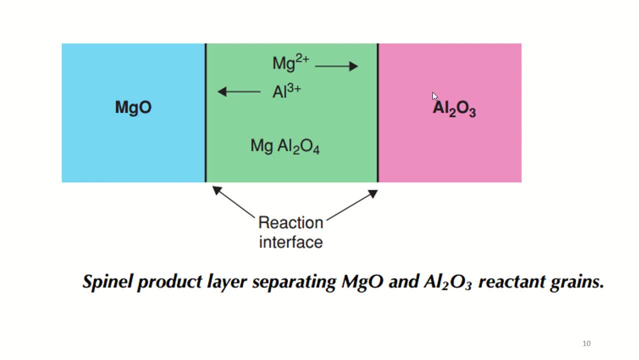 Using We Are Using Here Is Magnesium Oxide And Aluminium Oxide Are No Longer In Contact, But They Are Separated From The Outer Diffusion. 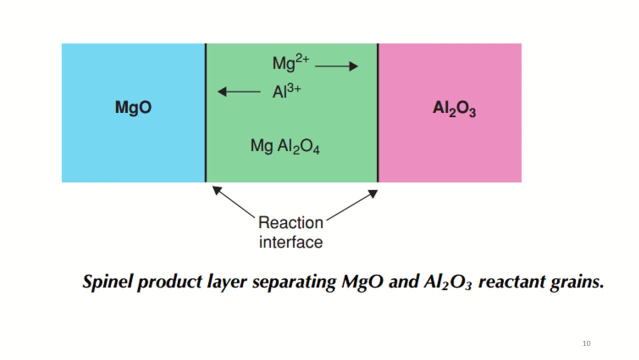 Process Is Then Required In Which Magnesium Mg2+ Ions Diffuse Away From An Aluminium 3+ Ions Diffuse Towards The Magnesium Oxide. 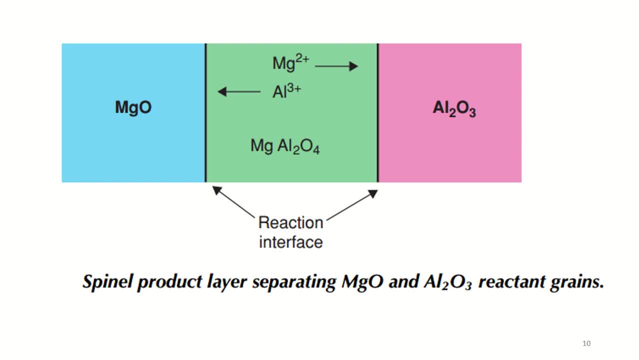 Magnesium- Aluminium Oxide Interface Is Quite Clear About The Interfaces Of Magnesium Oxide And Aluminium Magnesium Oxide Interfaces Because Complex Counter Diffusion. 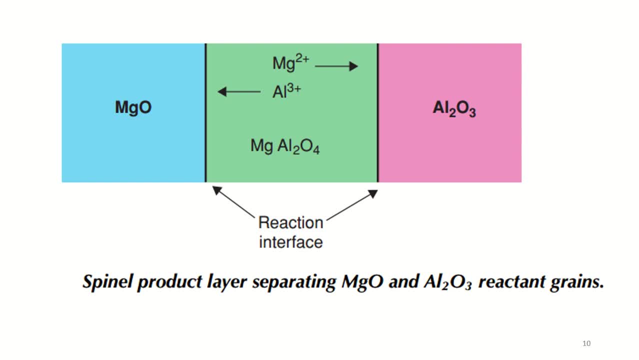 Process Is Supposed To Be Required, In Which The Magnesium Mg2+ Ions Diffuse Towards The Magnesium Oxide, As Well As Magnesium Aluminium.